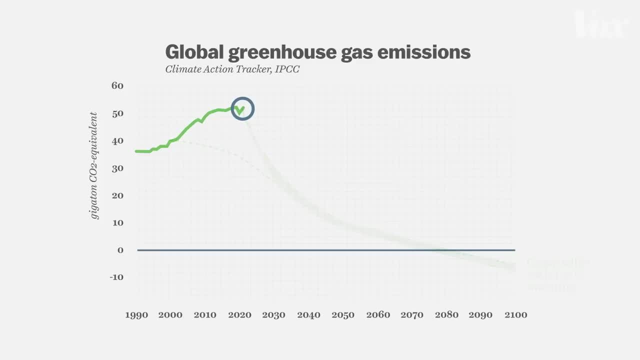 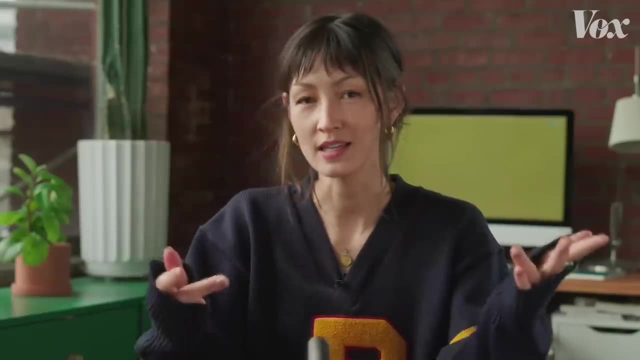 now we're up here and the math is getting really tough. So to make it work, governments are penciling in negative emissions. That's the net part of the net zero promise, the idea that we're cutting emissions, That we can reach zero while still emitting greenhouse gases if we're also taking CO2. 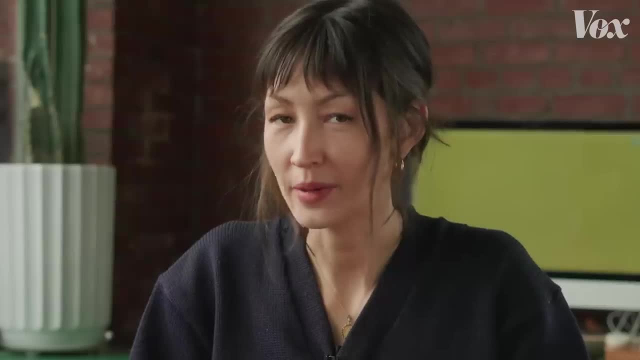 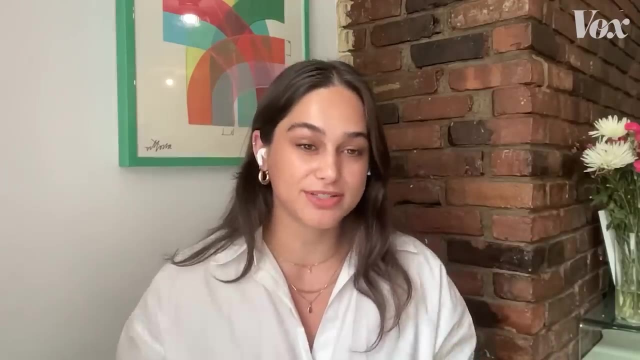 out of the air. It's a bit contentious, but we're going to be hearing a lot about it. It's called CDR, so carbon dioxide removal. What we want to do is put that carbon back where it belongs. Gianna Amador is a CDR advocate and she's going to help us explain this with the bathtub. 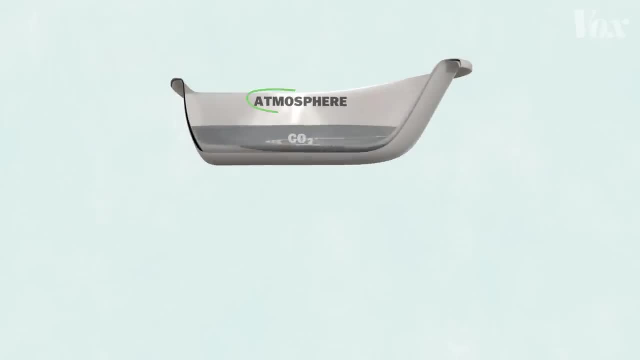 metaphor: The bathtub in this situation is our atmosphere and the water in the bathtub is the CO2 that's in our atmosphere. Before the Industrial Revolution, the land and ocean typically released as much CO2 into the air as they absorbed back down through. 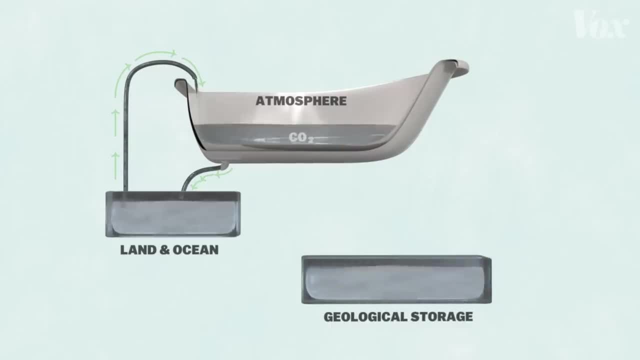 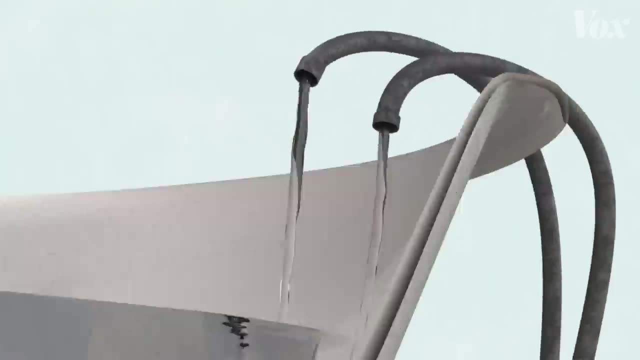 this drain, But when people started digging up coal and oil to power their machines, first in Europe and then in the US, it sent this new flow of CO2 into the air, one that the plants and oceans couldn't keep up with. About 45% of those emissions stay in the atmosphere. 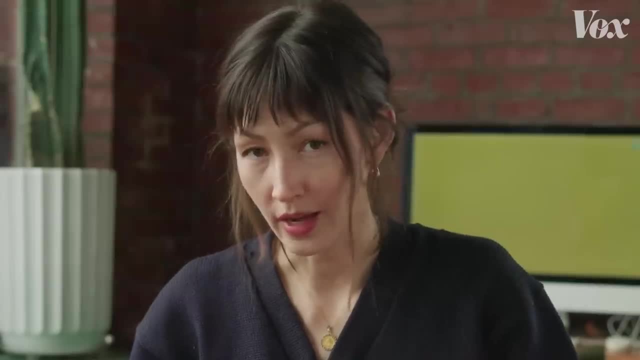 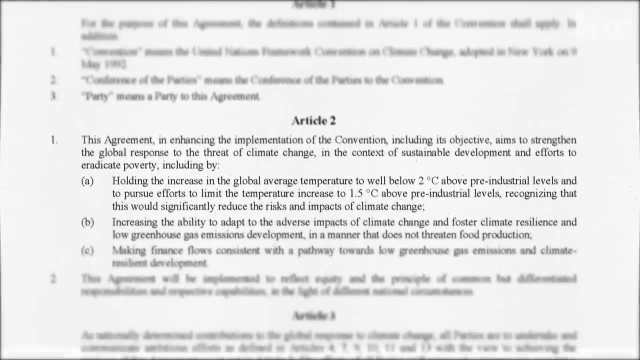 trapping heat and setting us up for an escalating array of climate disasters. So in 2015,, all of the countries sent someone off to pick up CO2.. We sent someone off to Paris to say: OK, everyone, we need to keep warming well below. 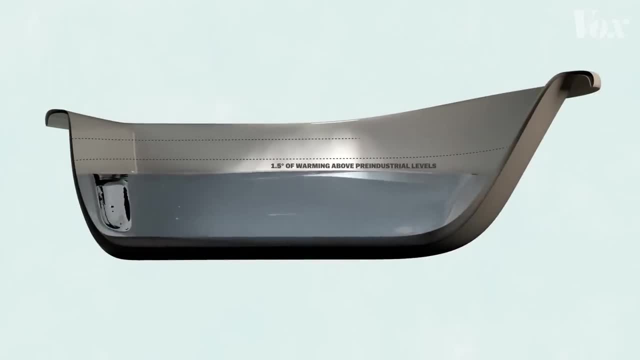 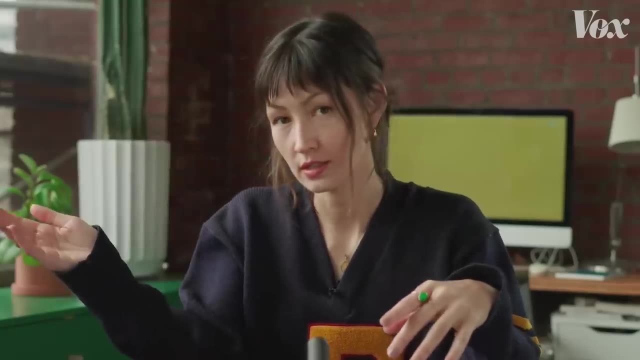 2 degrees Celsius, And really we're aiming for 1.5 degrees. That's above pre-industrial levels, And the exact numbers matter less than the fact that every increment of warming increases risk. So, first and foremost, we need to turn off the tap. Everything else is futile if we don't. 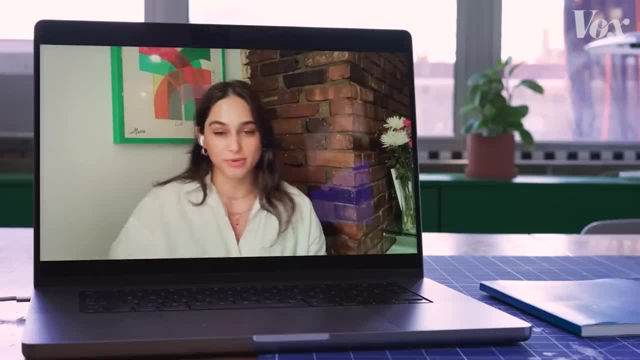 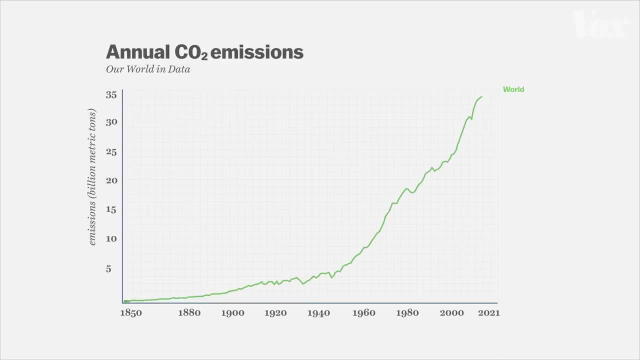 stop the root of the problem today. Turn off that tap, stop emitting CO2.. Not only have we not turned off any taps: global emissions are still rising, especially in Asia, where 60% of human beings live, many of whom are just emerging out of poverty. 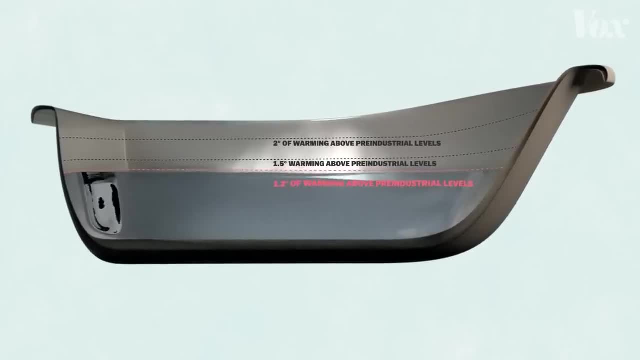 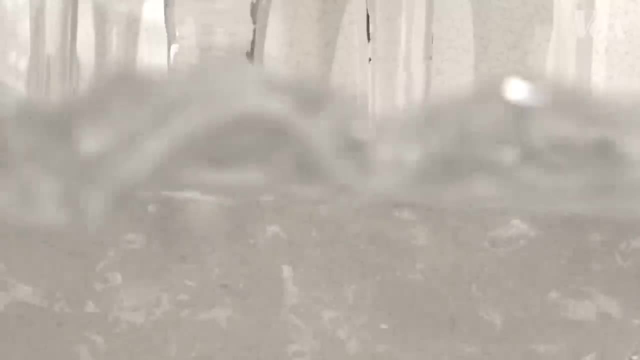 So now we're here at nearly 1.2 degrees of warming. Frankly, we have not done what it would take to meet that 1.5-degree goal, But we may be able to keep warming under 2 degrees if all of those net-zero promises become real net-zero policies. And that's where things 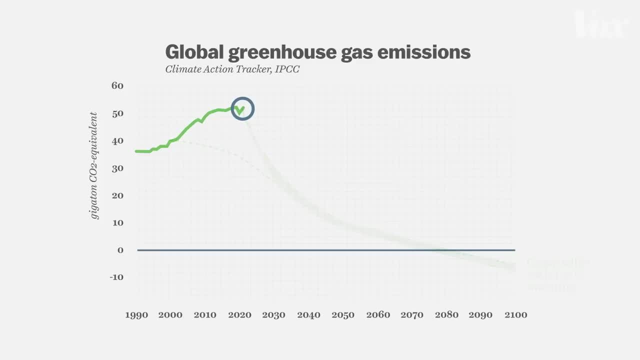 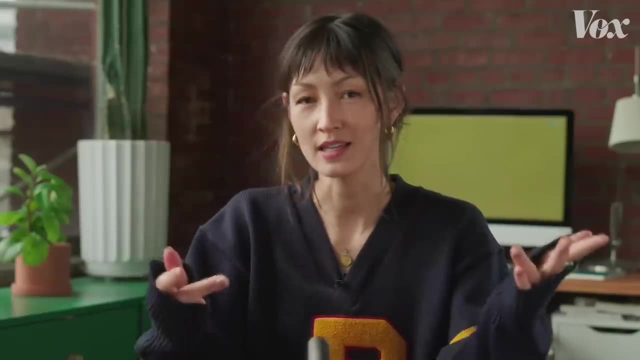 now we're up here and the math is getting really tough. So to make it work, governments are penciling in negative emissions. That's the net part of the net zero promise, the idea that we're cutting emissions, That we can reach zero while still emitting greenhouse gases if we're also taking CO2. 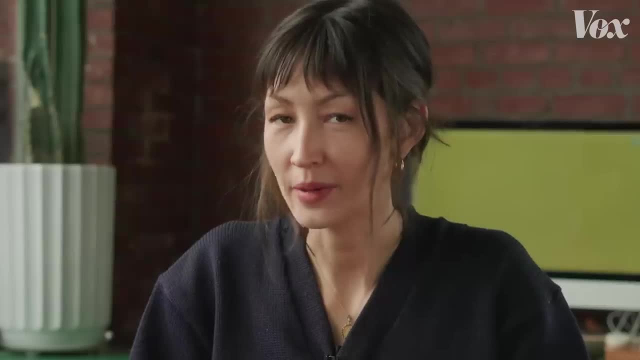 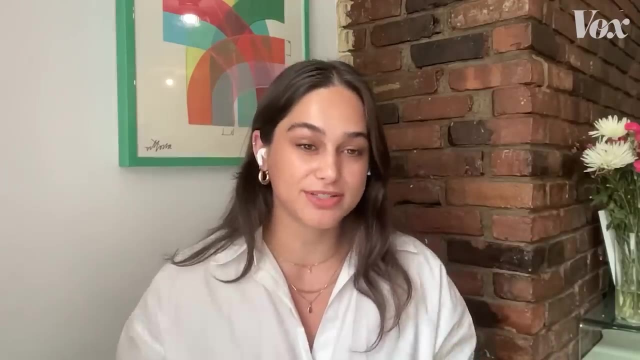 out of the air. It's a bit contentious, but we're going to be hearing a lot about it. It's called CDR, so carbon dioxide removal. What we want to do is put that carbon back where it belongs. Gianna Amador is a CDR advocate and she's going to help us explain this with the bathtub. 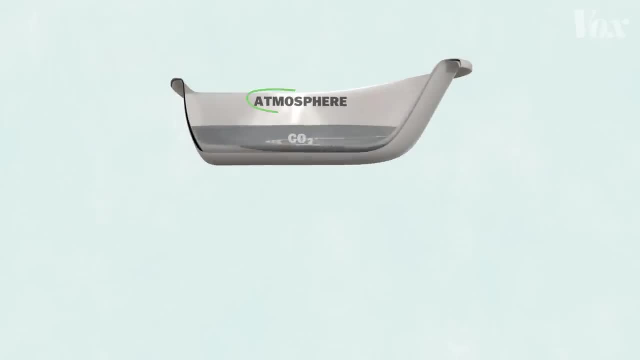 metaphor: The bathtub in this situation is our atmosphere and the water in the bathtub is the CO2 that's in our atmosphere. Before the Industrial Revolution, the land and ocean typically released as much CO2 into the air as they absorbed back down through. 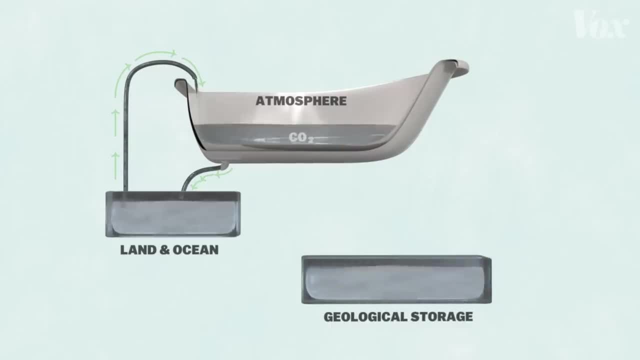 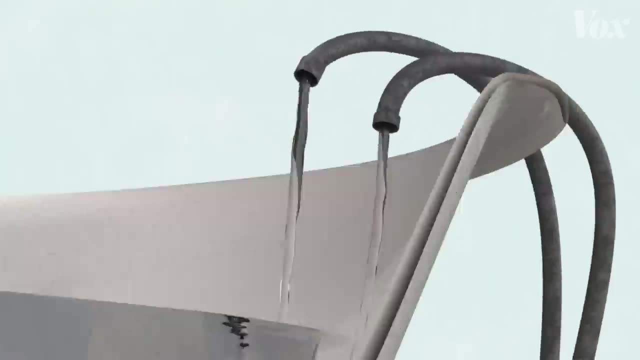 this drain, But when people started digging up coal and oil to power their machines, first in Europe and then in the US, it sent this new flow of CO2 into the air, one that the plants and oceans couldn't keep up with. About 45% of those emissions stay in the atmosphere. 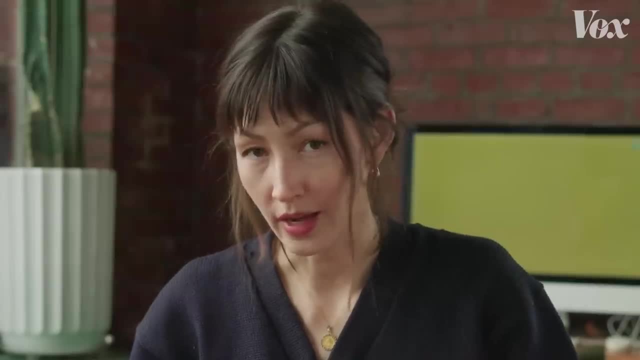 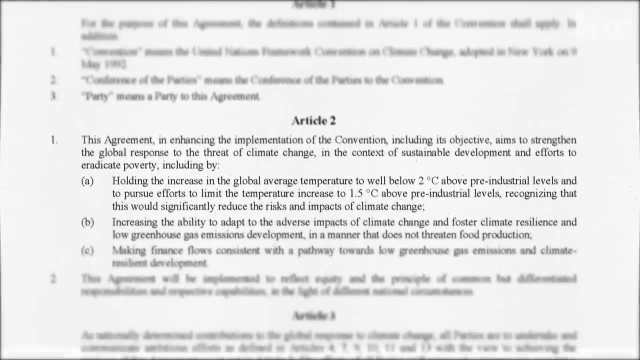 trapping heat and setting us up for an escalating array of climate disasters. So in 2015,, all of the countries sent someone off to pick up CO2.. We sent someone off to Paris to say: OK, everyone, we need to keep warming well below. 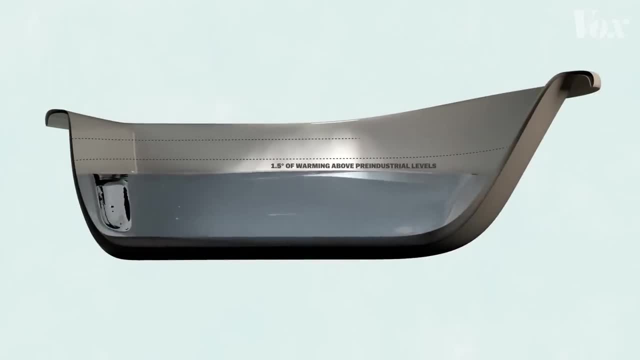 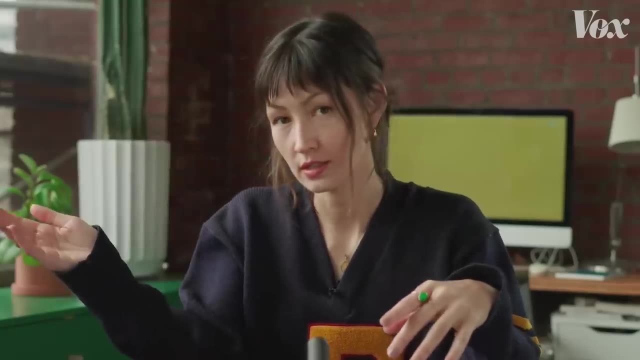 2 degrees Celsius, And really we're aiming for 1.5 degrees. That's above pre-industrial levels, And the exact numbers matter less than the fact that every increment of warming increases risk. So, first and foremost, we need to turn off the tap. Everything else is futile if we don't. 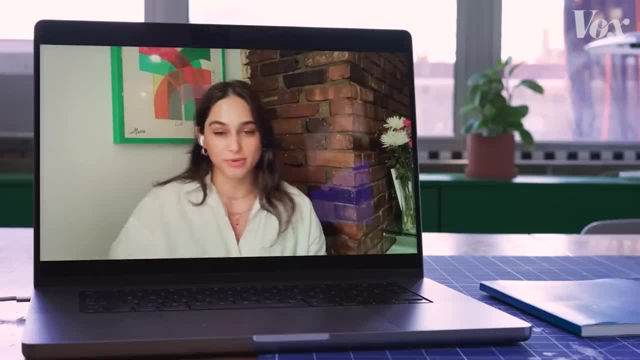 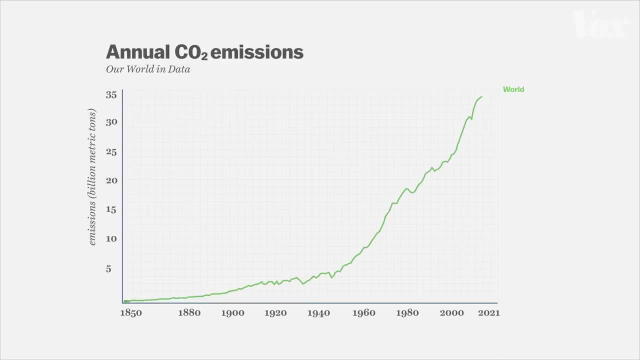 stop the root of the problem today. Turn off that tap, stop emitting CO2.. Not only have we not turned off any taps: global emissions are still rising, especially in Asia, where 60% of human beings live, many of whom are just emerging out of poverty. 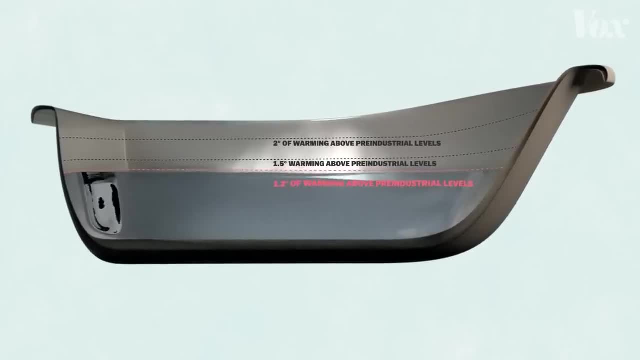 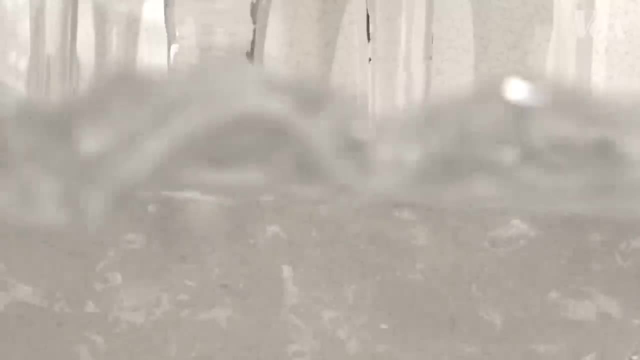 So now we're here at nearly 1.2 degrees of warming. Frankly, we have not done what it would take to meet that 1.5-degree goal, But we may be able to keep warming under 2 degrees if all of those net-zero promises become real net-zero policies. And that's where things 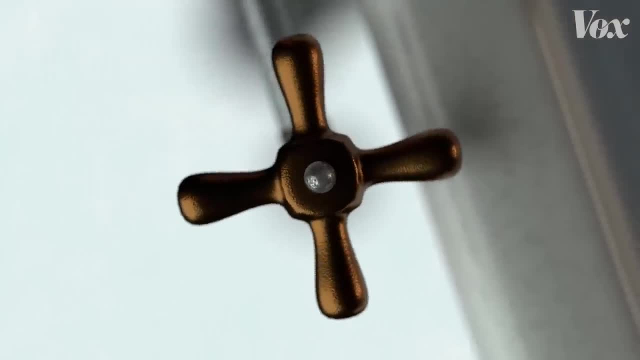 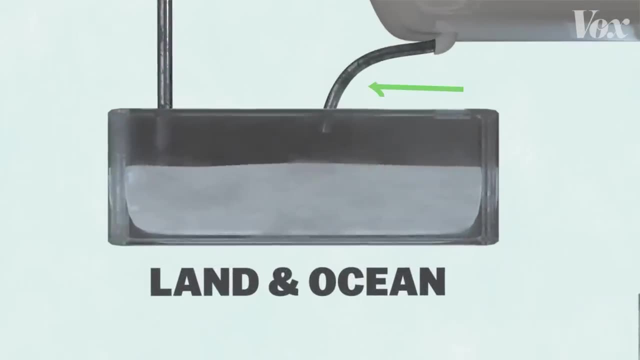 get a little tricky. Turning these emissions all the way off could get really hard, really expensive or even unbearable. So everyone's kind of hoping that we can work from the bottom of the tub too To kind of increase the size of the drain, increase the speed in which we can drain that. 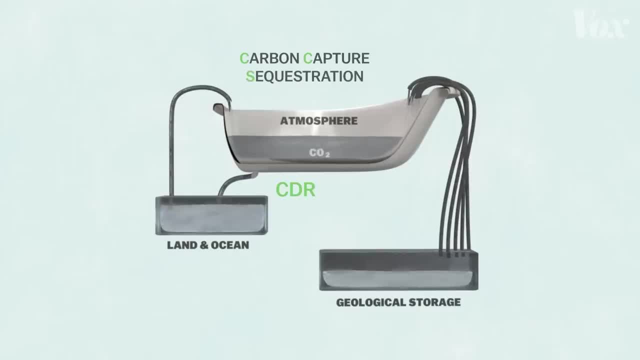 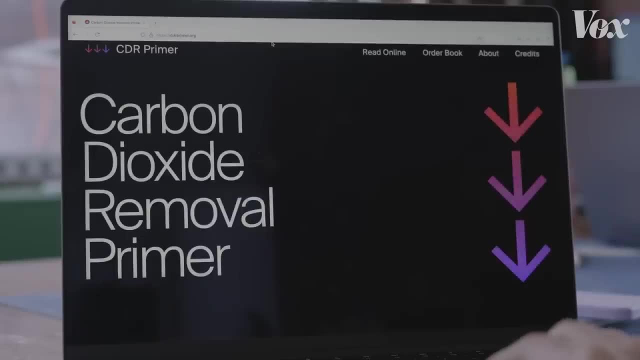 water from the bathtub. Now, CDR is distinct from CCS, which prevents emissions at the source That works on the faucet. CDR grabs CO2 from the air, and people have come up with a lot of interesting ways of doing that. The most common one so far is planting and protecting forests. It's one. 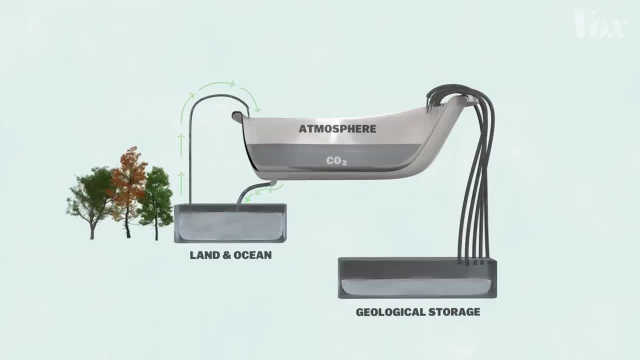 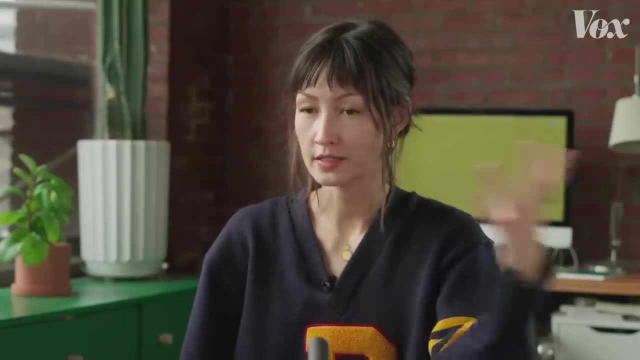 of the more affordable CDR approaches right now and it has a lot of benefits aside from capturing CO2.. But we've seen from problems with the carbon offsets market that it can be hard to verify And you know, trees don't live forever. So most of the modeling scenarios that limit warming assume we'll. 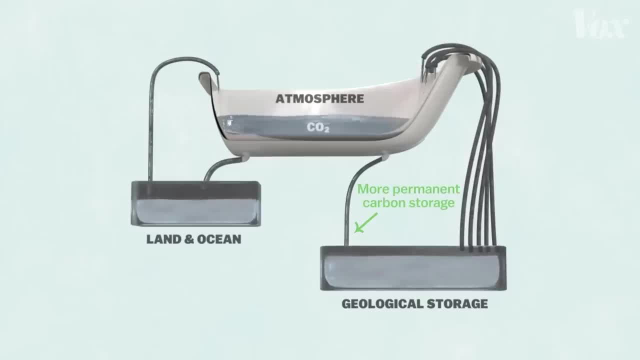 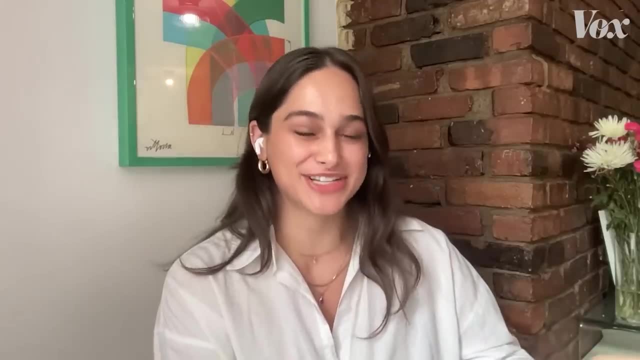 also be able to build a new drain for more permanent carbon storage. So through things like rock weathering, we can crush up a bunch of rocks that naturally react with CO2 and try to speed up that reaction, Or we can use chemistry to mimic natural processes. 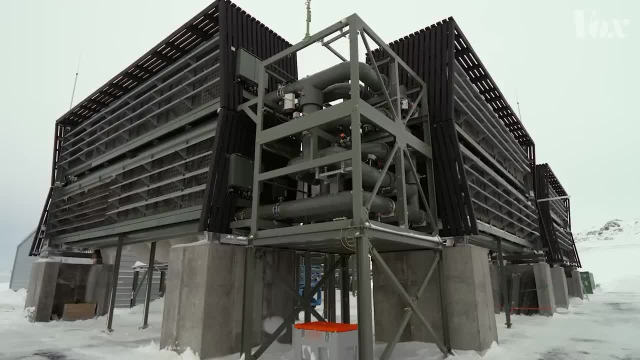 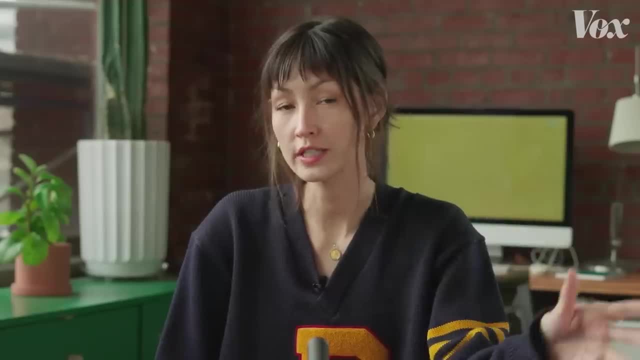 through technologies like direct air capture, which basically use a type of chemical that selectively binds with CO2 to capture it from the air. These techniques all come with different costs and they're in really early stages of development, So there's a concern that the people in charge of the faucets will see any movement down. 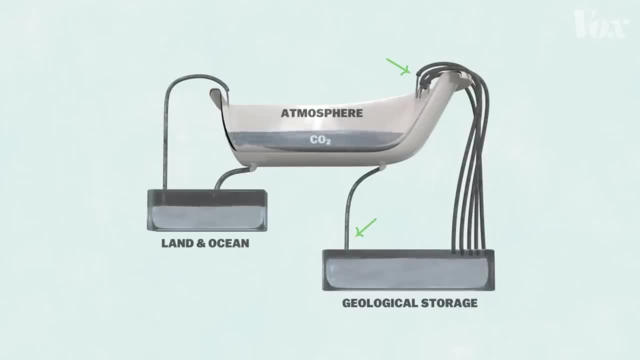 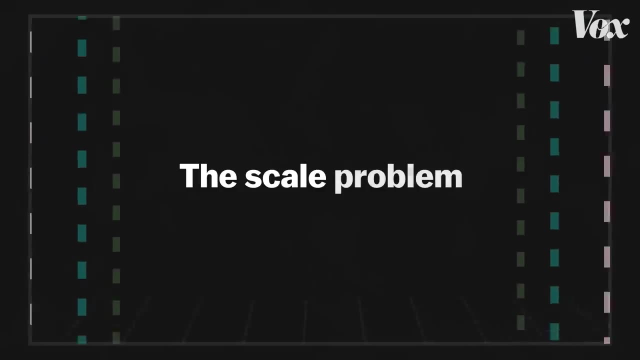 here as an excuse to avoid making cuts up there. Should we be counting on large amounts of carbon removal for our climate plans? Well, it seems we already are. The US government's net-zero plan calls for 500 million metric tons of CO2 removal by 2050.. Up 4 billion tons. 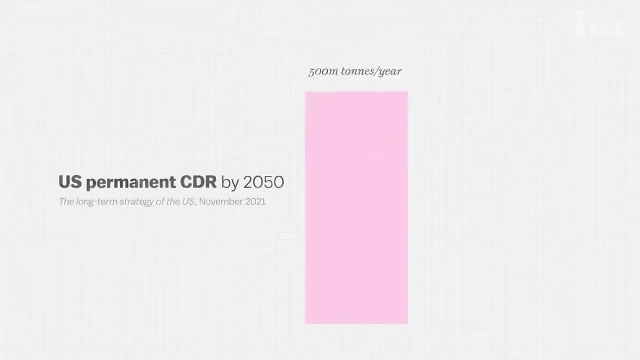 That's a lot. That's a lot, That's a lot. Up from zero today, Model simulations that limit warming to 1.5 degrees envision around 3.8 billion tons of permanent carbon removal globally every year, And this is the 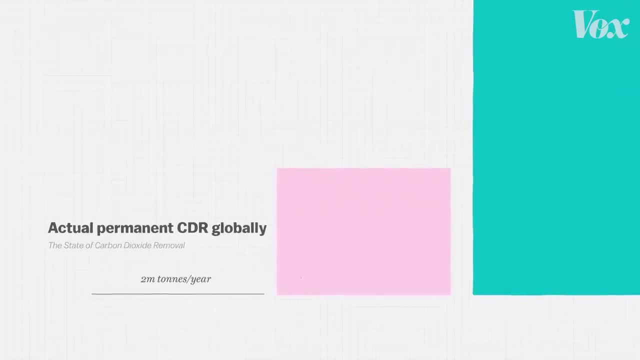 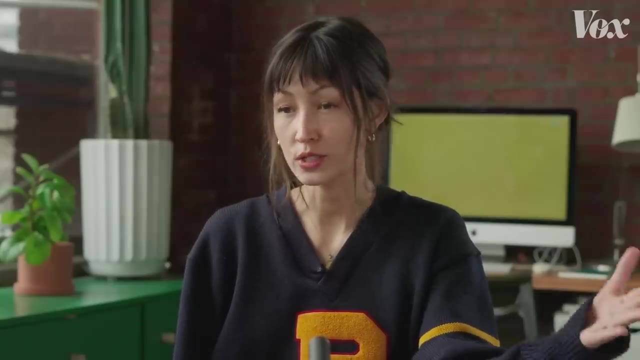 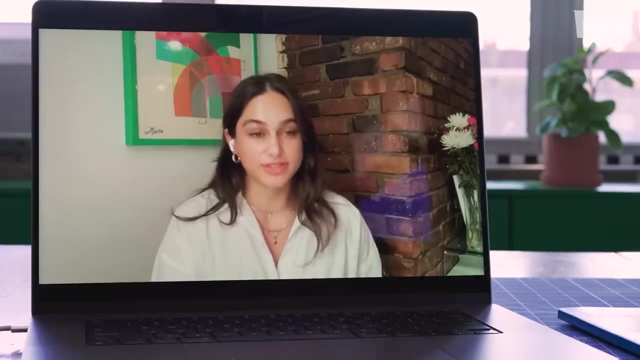 total amount of permanent carbon removal that has happened so far. So would you call that wishful thinking Or is it foresight about how much can happen in 30 years if we start our way up the learning curve now, We have actually a really strong playbook of developing technologies and driving down. 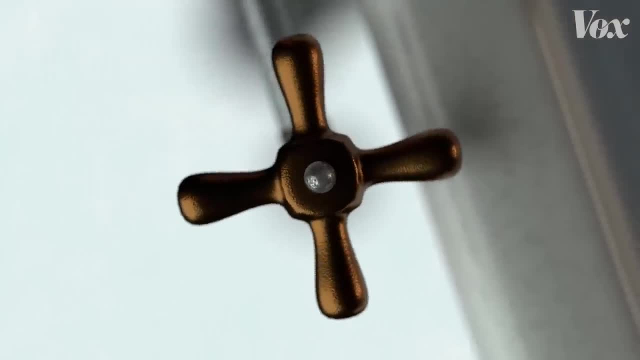 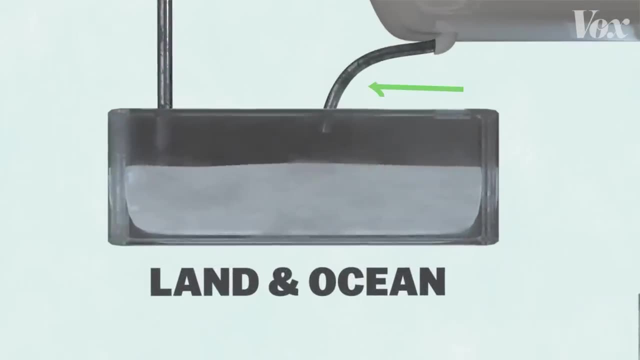 get a little tricky. Turning these emissions all the way off could get really hard, really expensive or even unbearable. So everyone's kind of hoping that we can work from the bottom of the tub too To kind of increase the size of the drain, increase the speed in which we can drain that. 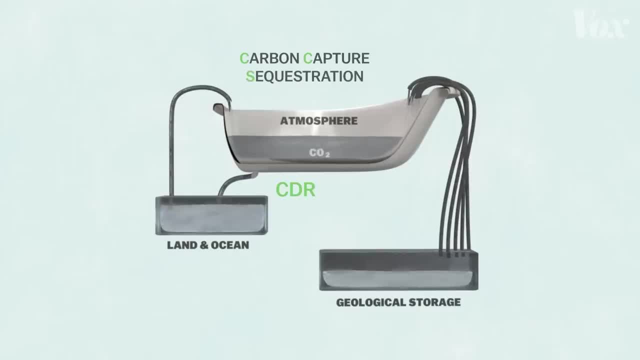 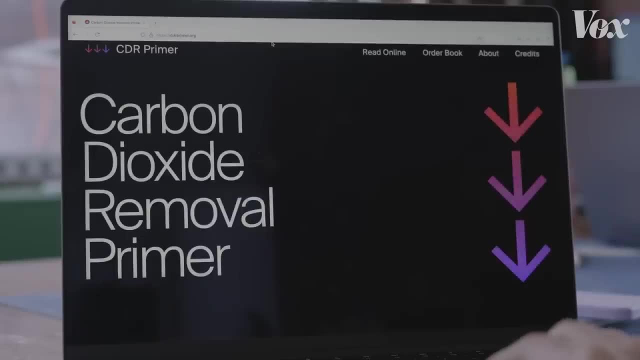 water from the bathtub. Now, CDR is distinct from CCS, which prevents emissions at the source That works on the faucet. CDR grabs CO2 from the air, and people have come up with a lot of interesting ways of doing that. The most common one so far is planting and protecting forests. It's one. 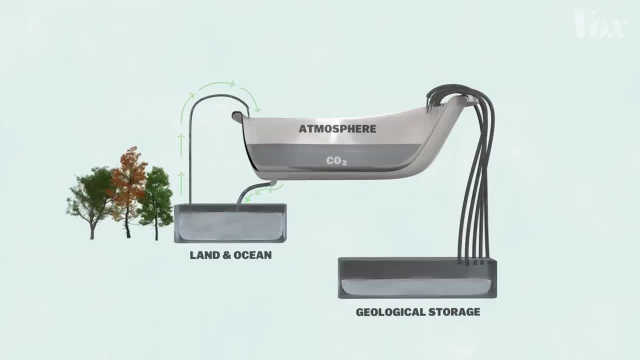 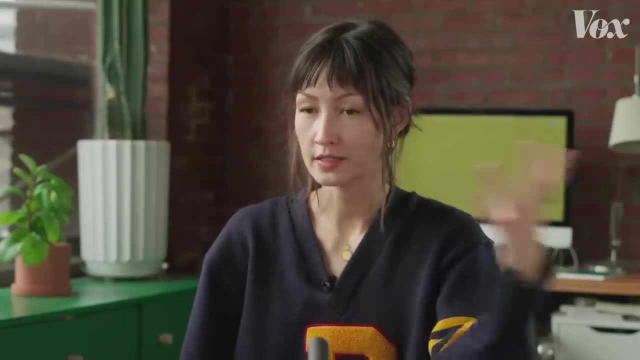 of the more affordable CDR approaches right now and it has a lot of benefits aside from capturing CO2.. But we've seen from problems with the carbon offsets market that it can be hard to verify And you know, trees don't live forever. So most of the modeling scenarios that limit warming assume we'll. 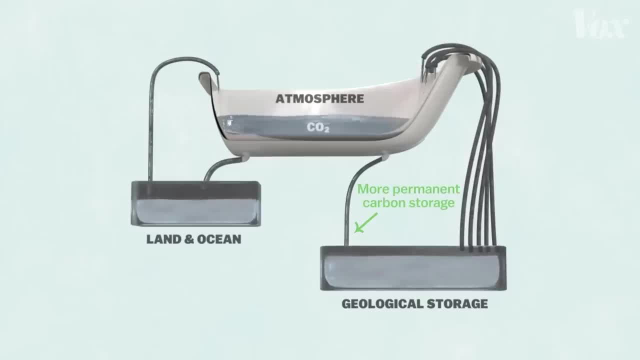 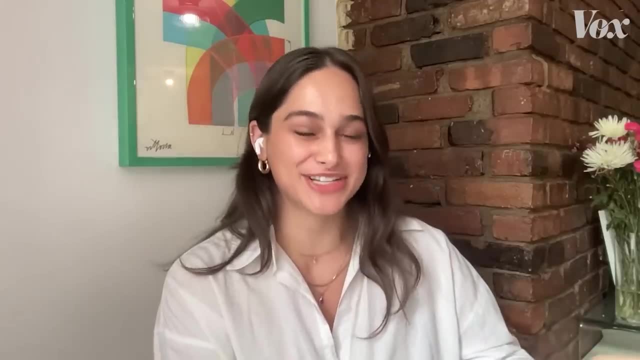 also be able to build a new drain for more permanent carbon storage. So through things like rock weathering, we can crush up a bunch of rocks that naturally react with CO2 and try to speed up that reaction, Or we can use chemistry to mimic natural processes. 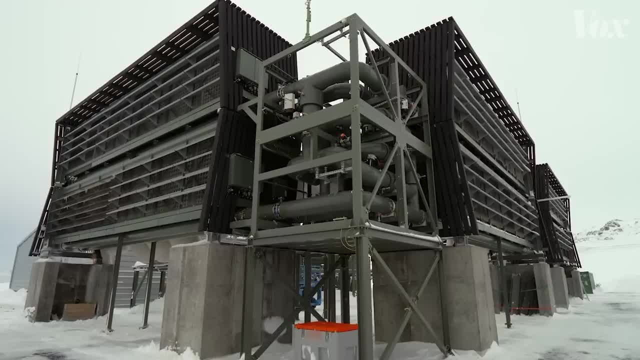 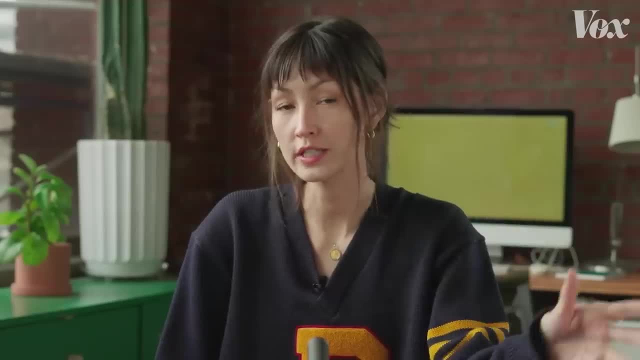 through technologies like direct air capture, which basically use a type of chemical that selectively binds with CO2 to capture it from the air. These techniques all come with different costs and they're in really early stages of development, So there's a concern that the people in charge of the faucets will see any movement down. 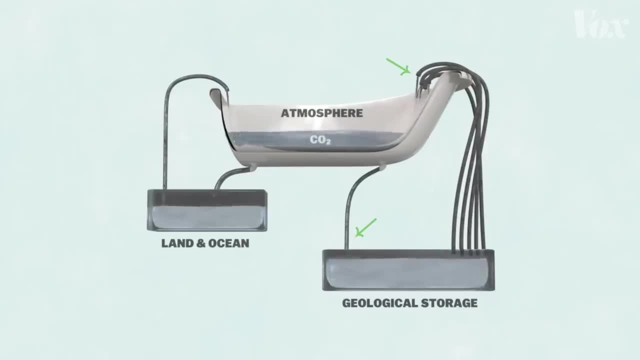 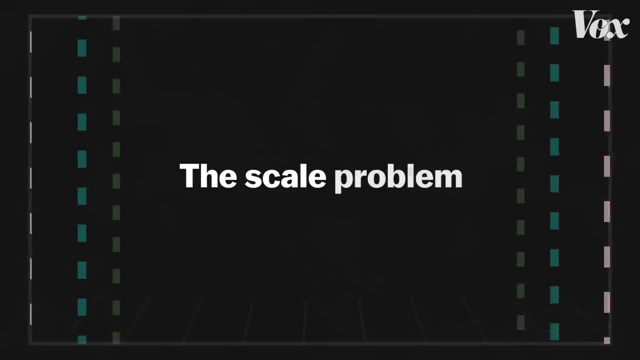 here as an excuse to avoid making cuts up there. Should we be counting on large amounts of carbon removal for our climate plans? Well, it seems we already are. The US government's Net Zero plan calls for 500 million metric tons of CO2 removal by 2050.. Up 4 million tons. 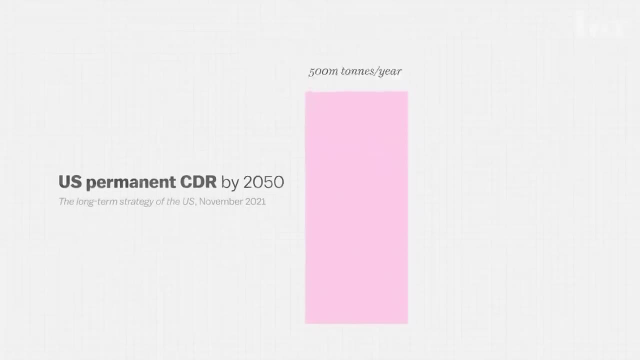 And that's a lot Up from zero. today, Model simulations that limit warming to 1.5 degrees envision around 3.8 billion tons of permanent carbon removal globally every year, And this is the total amount of permanent carbon removal that has happened so far. 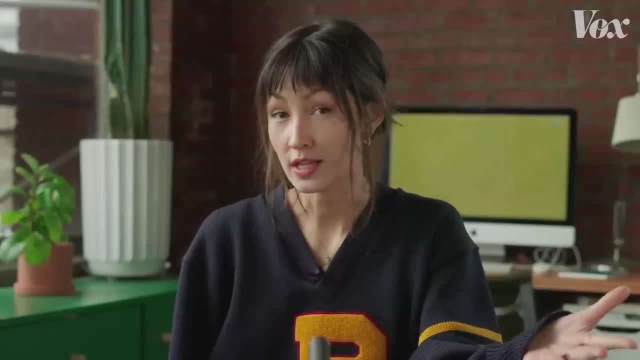 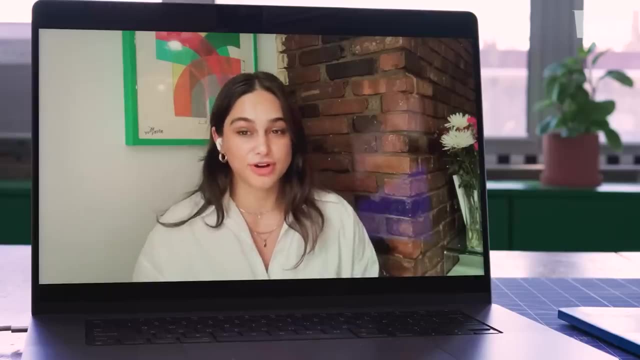 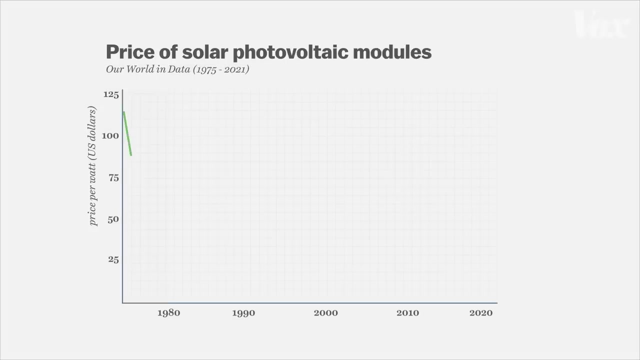 So would you call that wishful thinking, Or is it foresight about how much can happen in 30 years if we start our way up the learning curve? now We have actually a really strong playbook of developing technologies and driving the driving down costs. If we go all the way back to the 1970s, we see technologies like